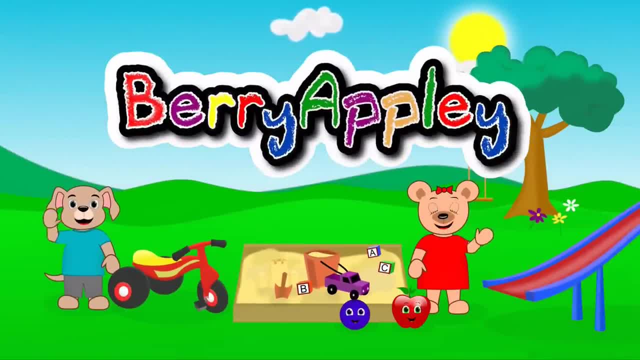 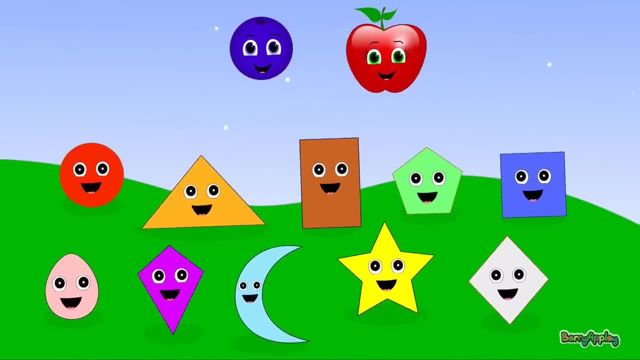 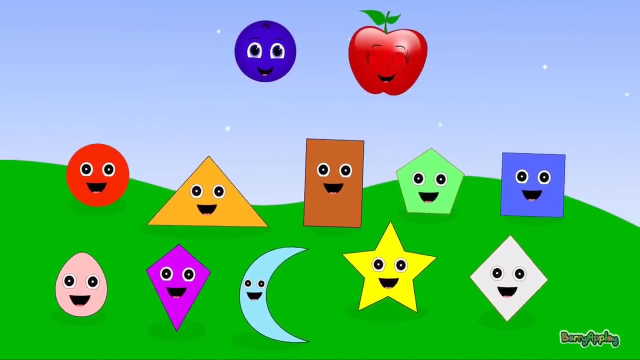 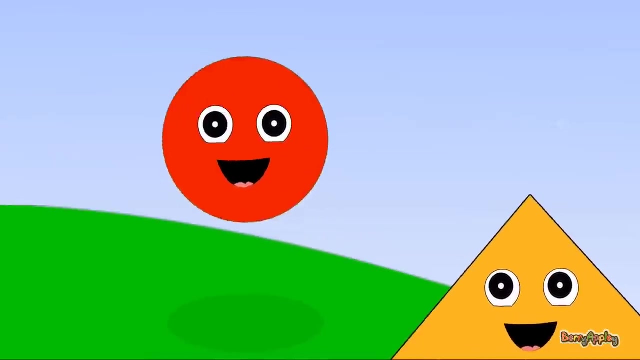 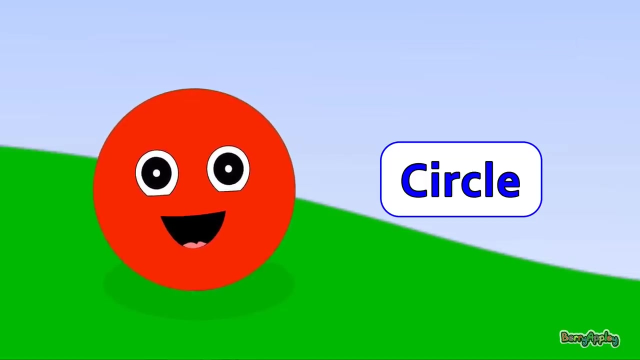 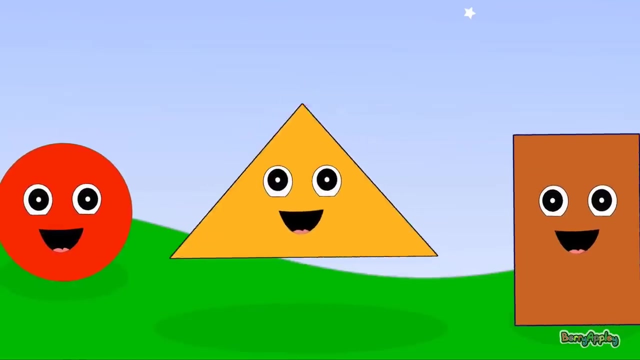 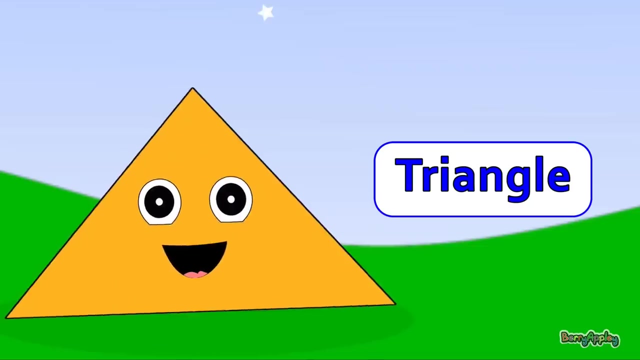 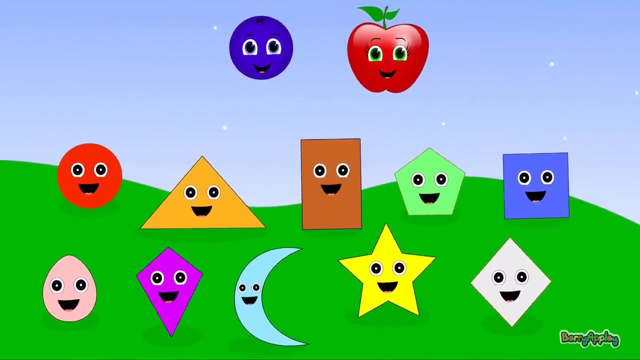 Play Appli Circle circle. where are you Here? I am here, I am. how do you do Circle, Circle, Triangle, triangle- where are you Here? I am, here, I am. how do you do Triangle, Triangle, Rectangle, rectangle- where are you? 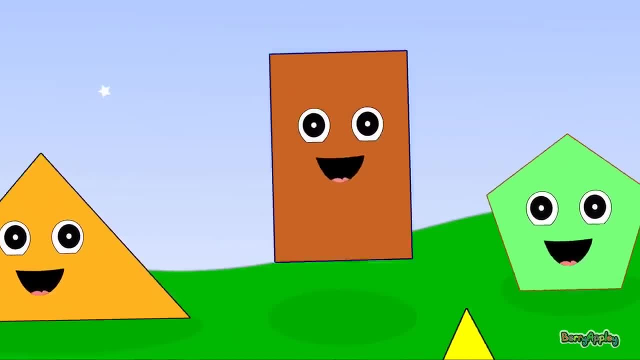 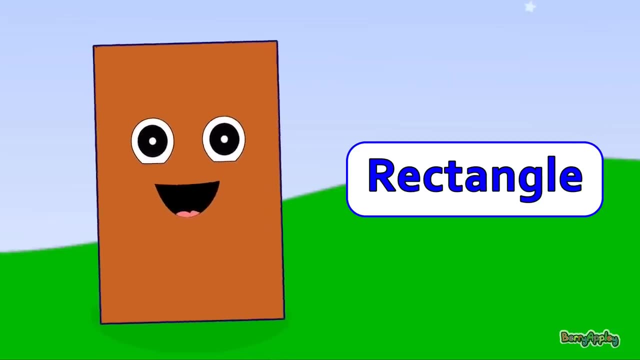 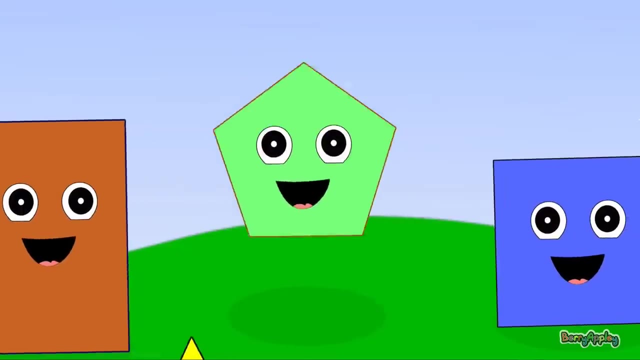 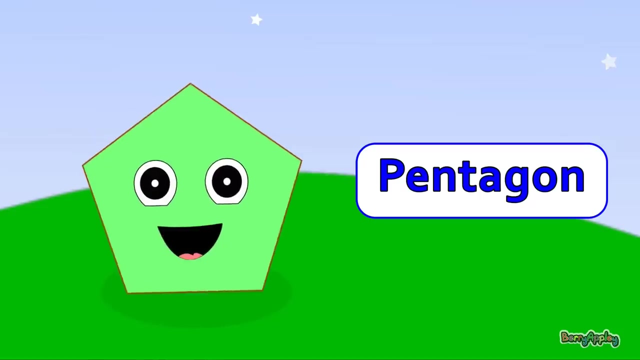 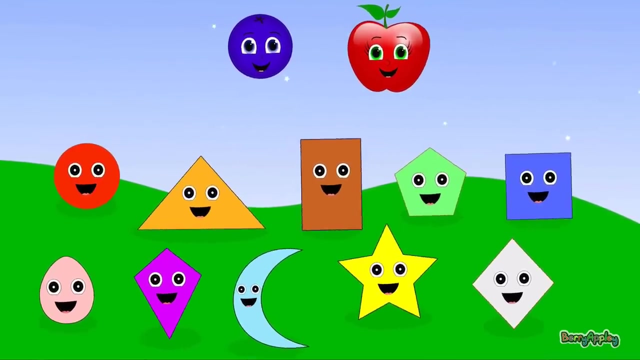 Here I am, here I am. how do you do? Rectangle, Rectangle, Pentagon, pentagon. where are you Here? I am, here I am. how do you do Pentagon, Pentagon, Square, square. where are you Here? I am, here I am. how do you do. 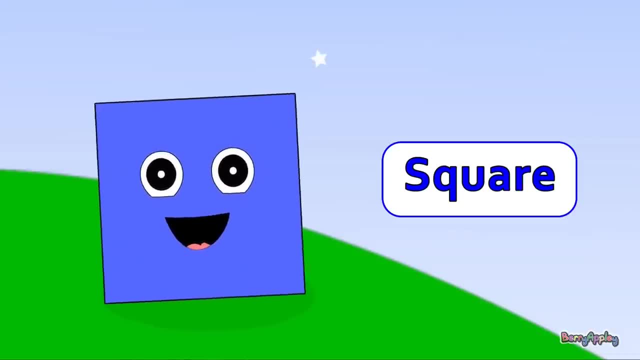 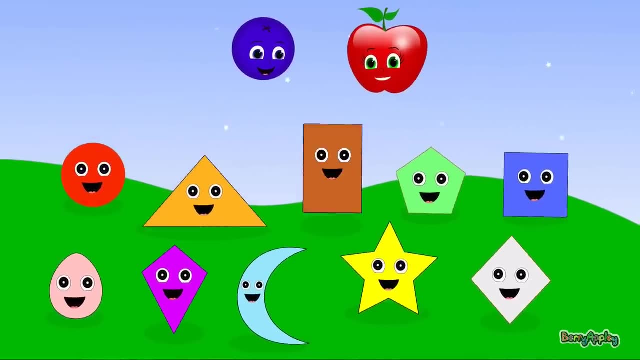 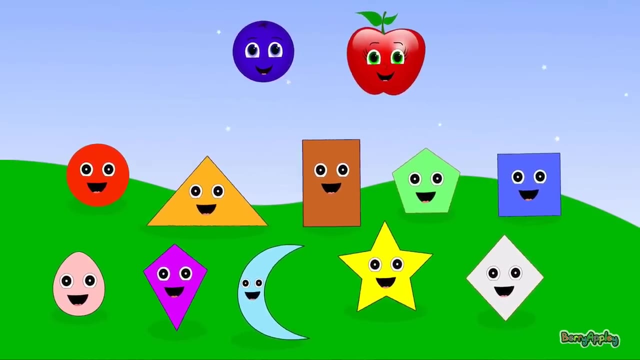 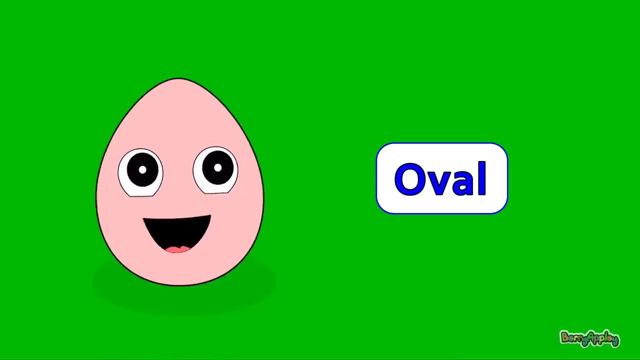 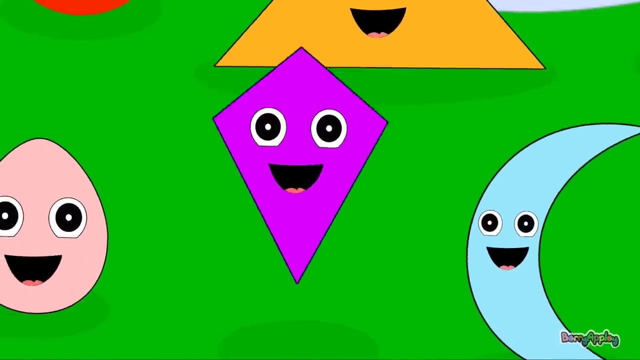 Square, Square Circle, Triangle, Rectangle, Pentagon Square, Oval oval. where are you Here? I am here, I am. how do you do? Oval Oval Kite kite. where are you Here? I am here, I am. how do you do. 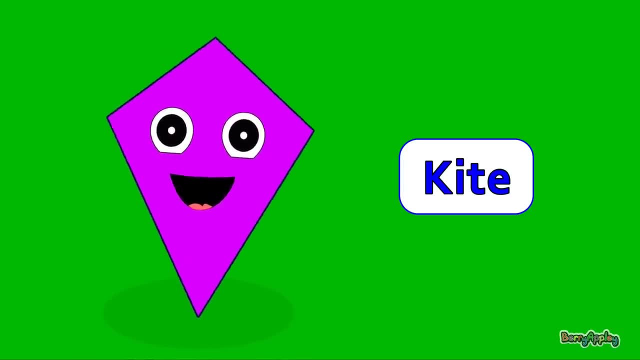 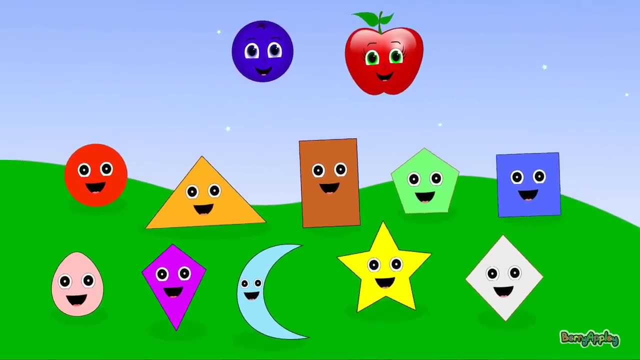 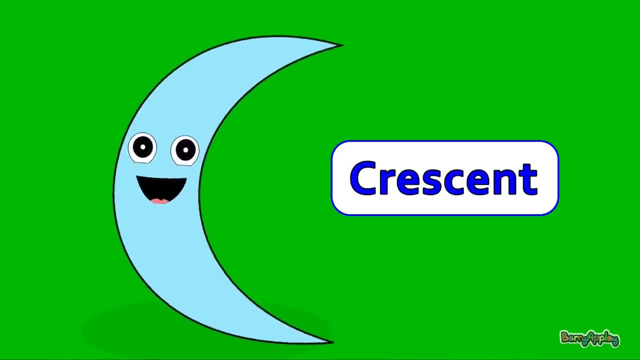 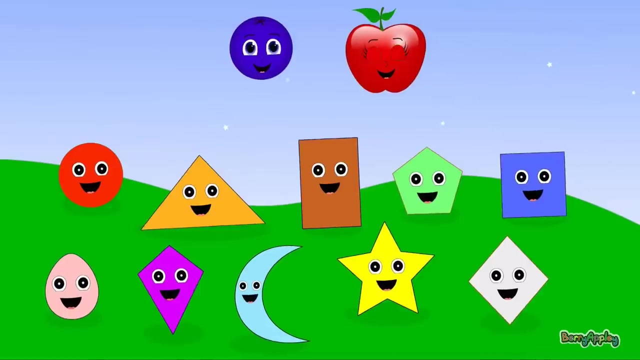 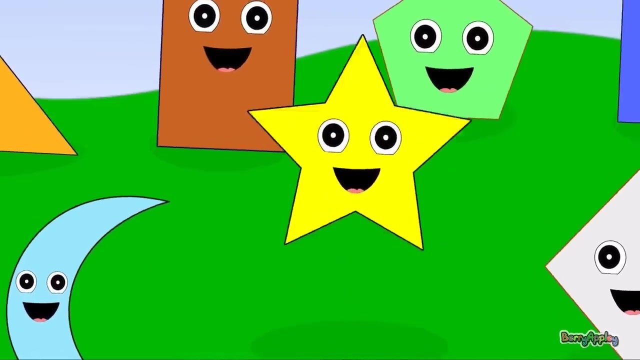 Kite, Kite, Crescent crescent. where are you Here? I am here, I am. how do you do Crescent Crescent Star star. where are you Here? I am here, I am. how do you do Star Star? 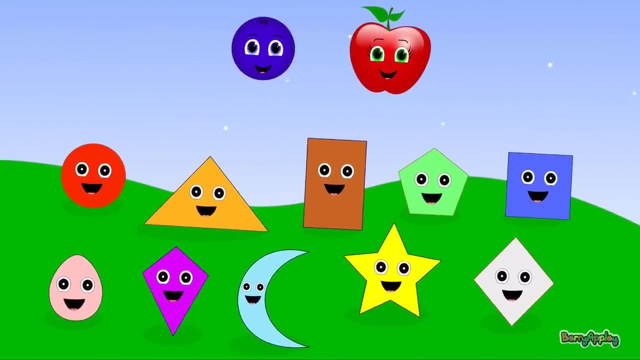 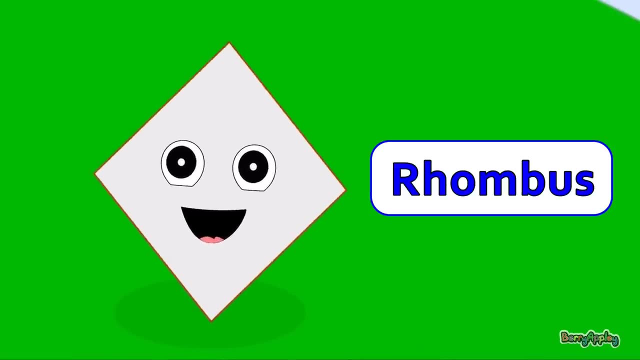 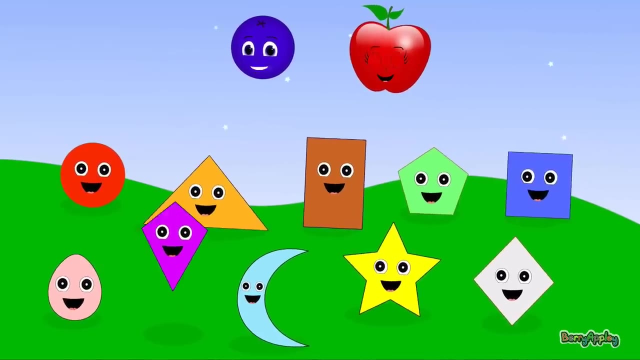 Rhombus rhombus. where are you Here? I am here, I am. how do you do Rhombus Rhombus? Rhombus, Oval, Oval, Kite, Crescent Star, Rhombus Shades, let's play hide and seek. 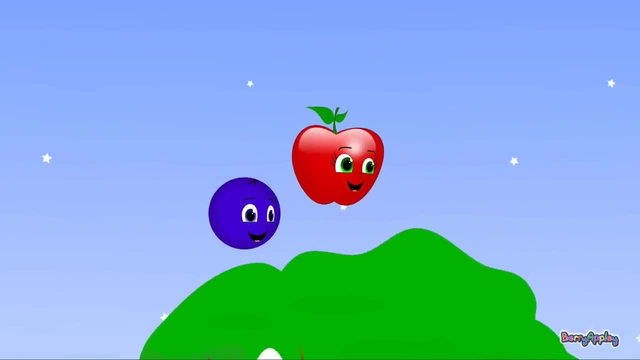 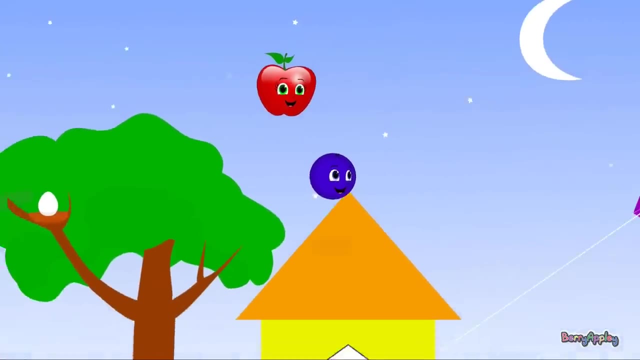 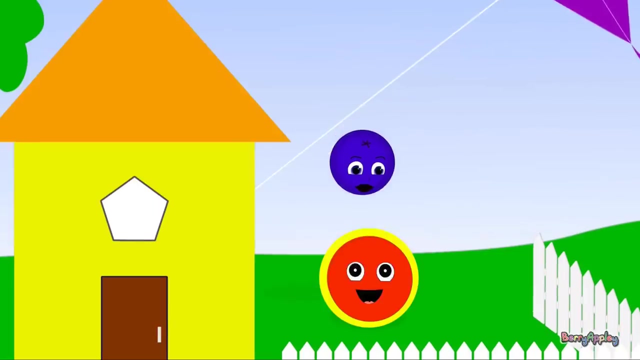 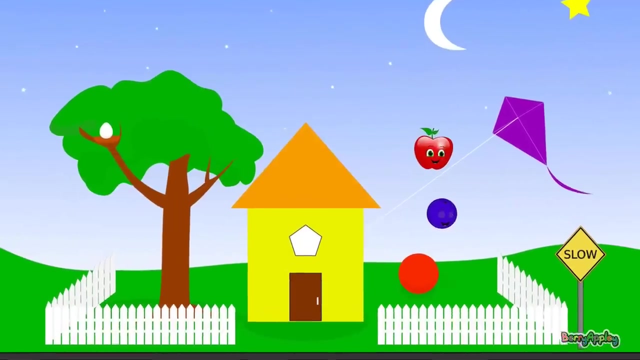 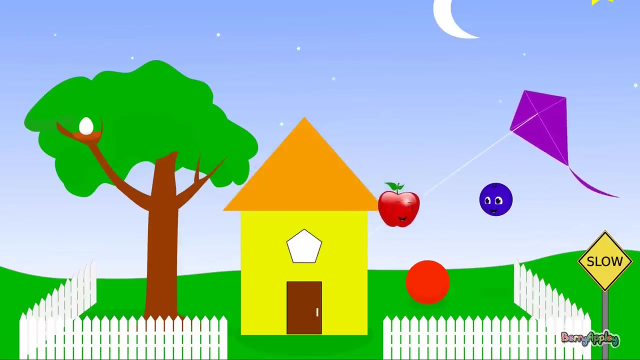 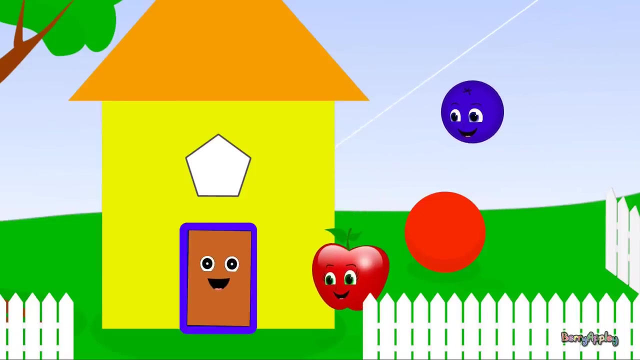 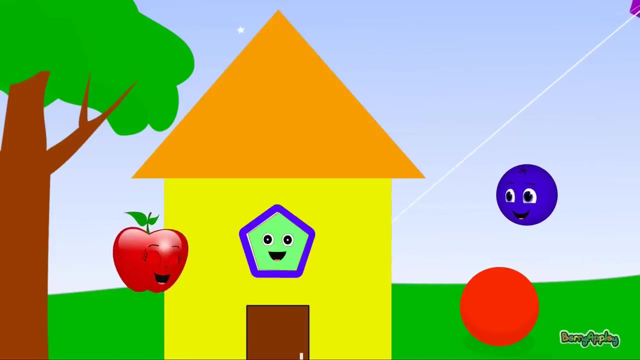 Yay, Let's find the shades. Yes, Can you find a circle, Circle, Circle, Good job. Can you find a triangle, Triangle, Triangle, Triangle, Very good. Can you find a rectangle Rectangle Rectangle- Great job, Great job. Can you find a pentagon Rectangle Rectangle. 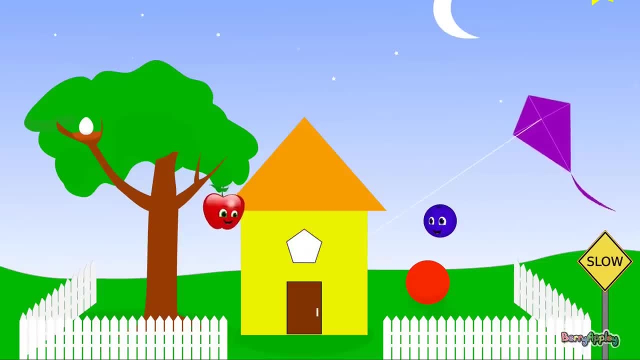 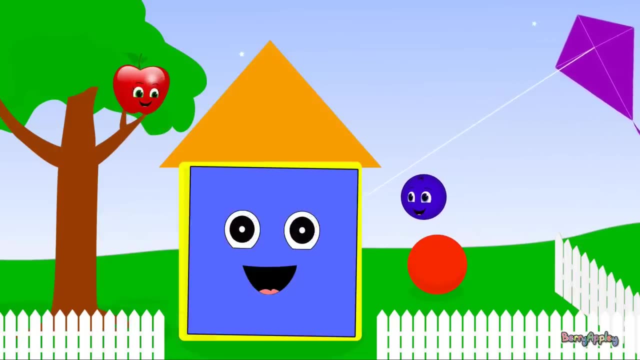 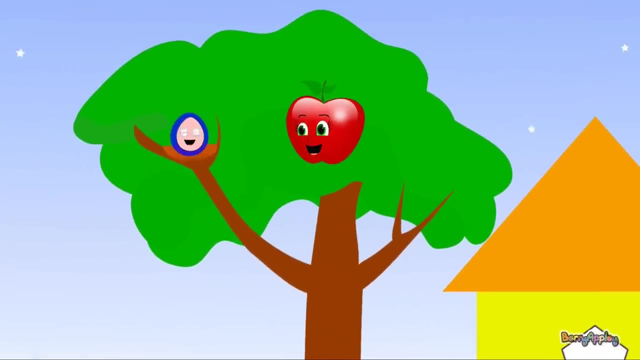 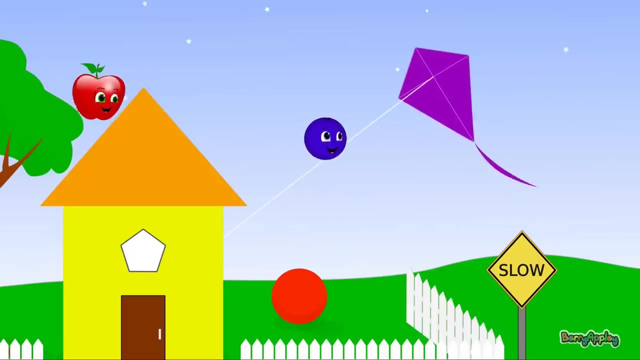 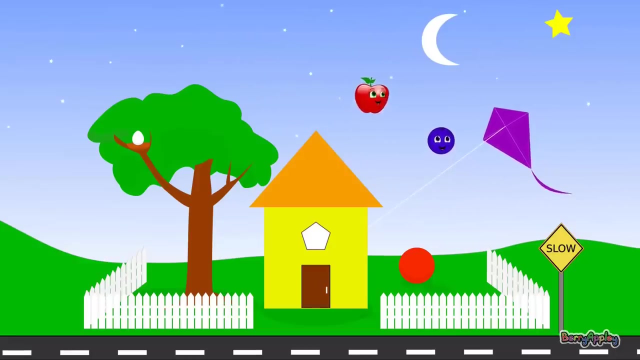 Rectangle, Great job. Can you find a square, Square, Square. You're so smart. Can you find an oval, Oval, Oval, Excellent. Can you find a kite, Kite, Kite, Great job. Can you find a crescent, Crescent, Crescent, Crescent. You're so smart Can you find a star. 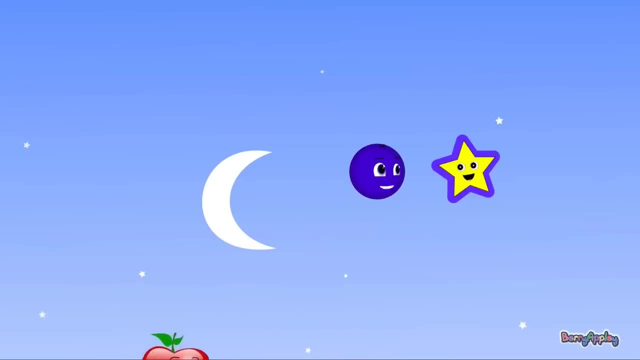 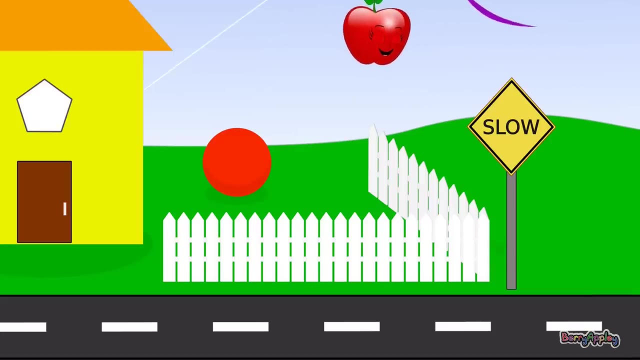 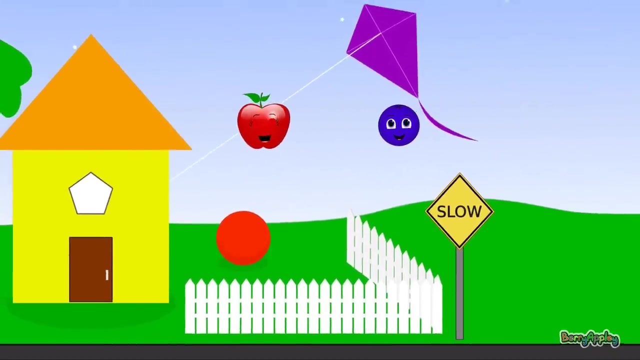 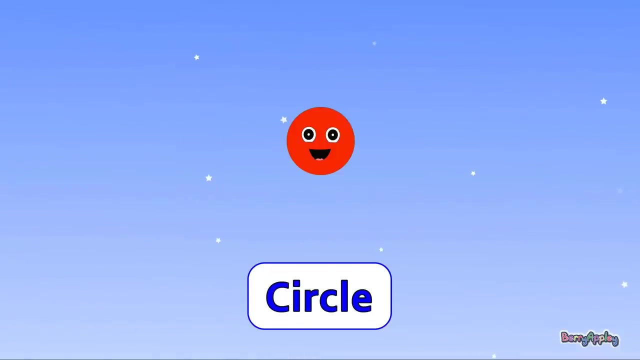 Star, Star, Excellent. Can you find a rhombus, Rhombus, Rhombus, You're smart. Yay, That was fun. Circle, Circle, Circle, Circle, Triangle, Triangle, Triangle, Triangle, Rectangle, Rectangle, Rectangle, Rectangle, Rectangle, Pentagon, Pentagon, Pentagon, Square, Square, Oval, Oval, Oval, Kite, kite, kite. 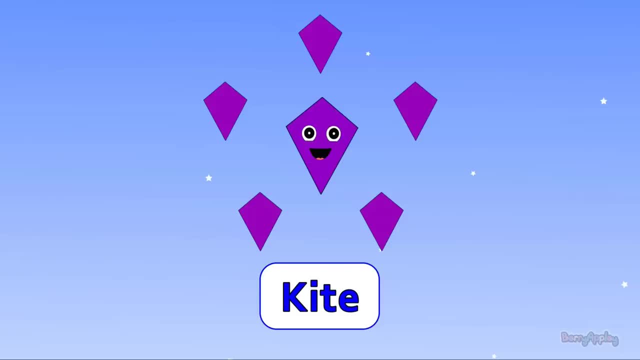 Kite, kite, kite Crescent crescent, crescent, Crescent, crescent crescent. Star, star, star, Star, star star. Rhombus rhombus rhombus, Rhombus, rhombus rhombus. 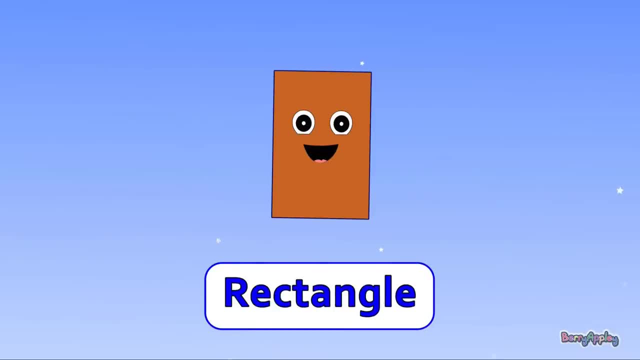 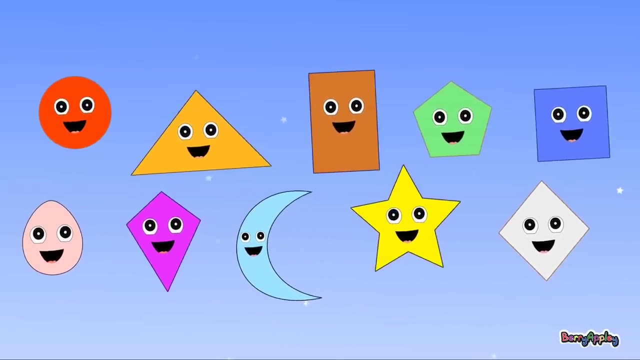 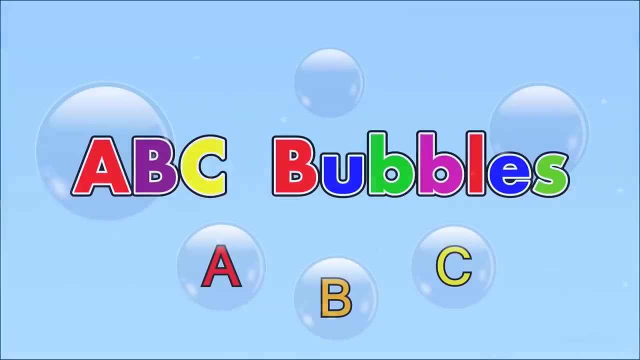 Circle, triangle, rectangle, Pentagon square, oval, Kite, crescent star, Rhombus. I like shapes. shapes are fun. Rainbow rainbow- rainbow A, B, C, D E, F G. A, B, C, D E, F G. 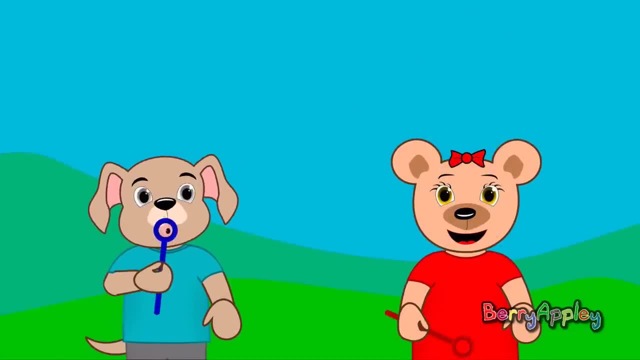 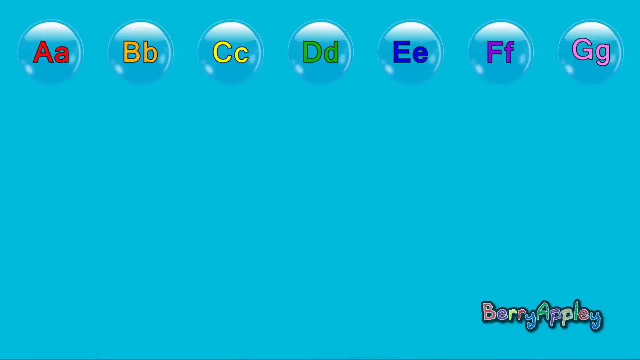 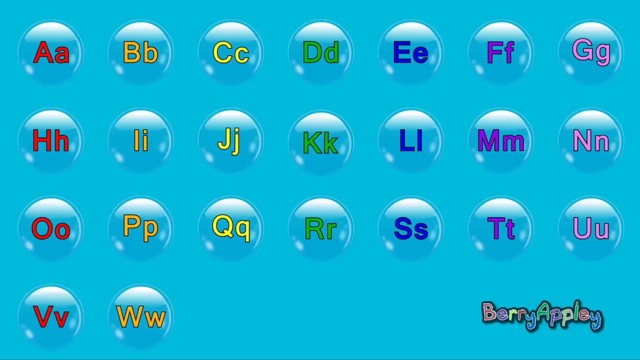 H, I J K L M N O P Q R S T U V W X Y Z Z R M N, W X Y Z A, B, C, D, E, F, G, H, I J K, L M N O P Q R S T U V W X Y Z. 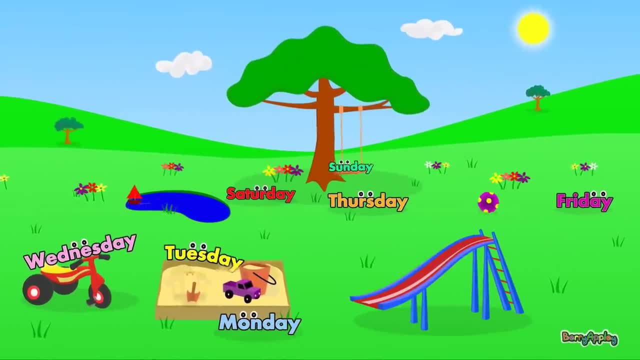 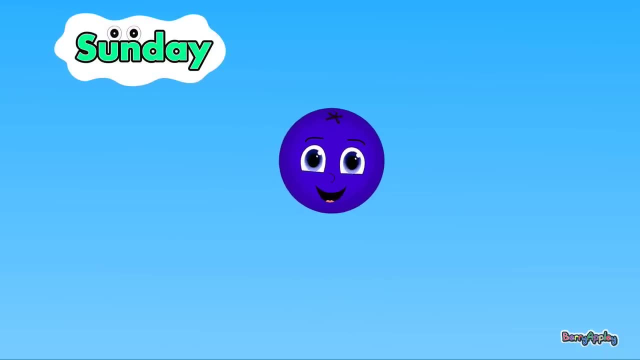 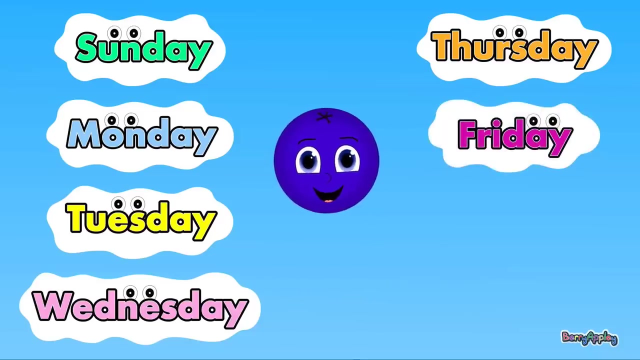 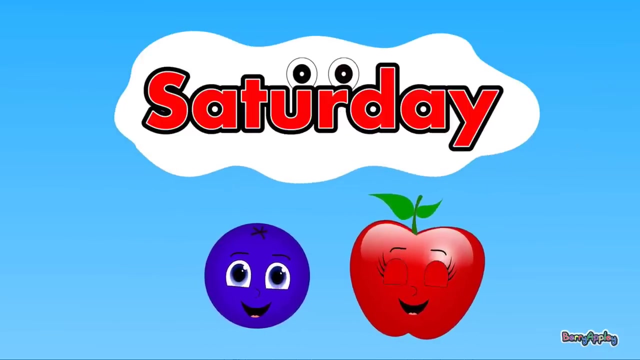 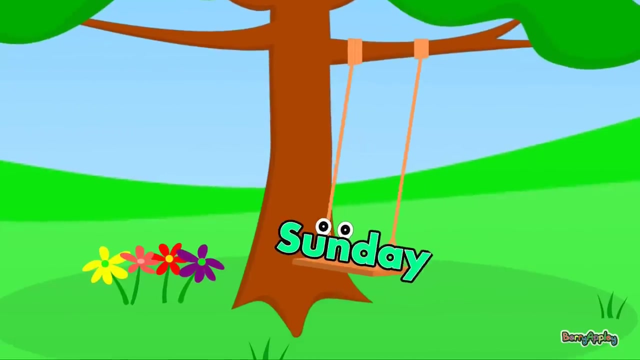 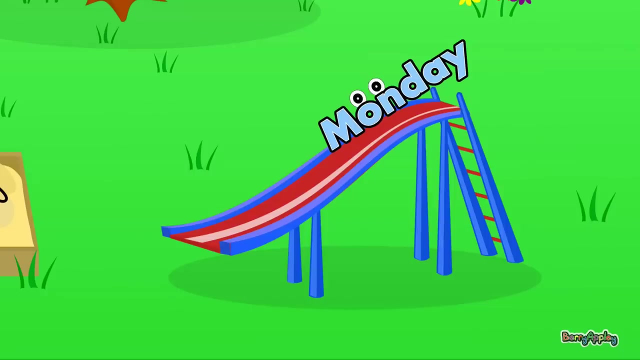 7 days of the week. 7 days of the week: Sunday, Monday, Tuesday, Wednesday, Thursday, Friday, Saturday, Sunday, Monday, Tuesday, Wednesday, Thursday, Friday, Saturday, Sunday, Sunday, Sunday, Sunday, Monday, Monday, Monday, Monday, Monday. 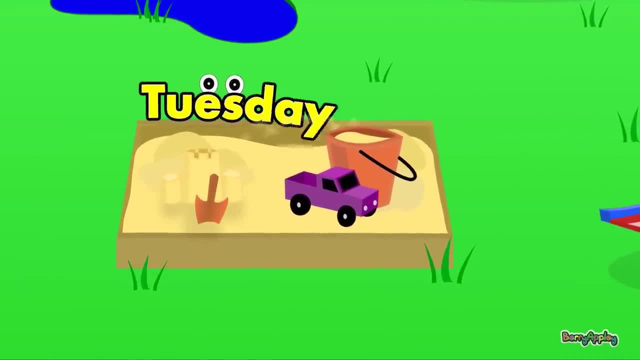 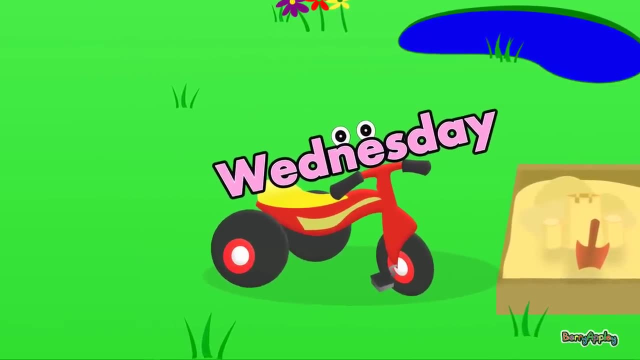 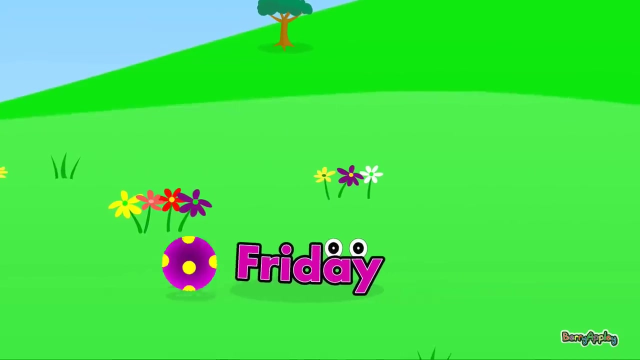 Tuesday, Tuesday, Tuesday, Tuesday, Wednesday, Wednesday, Wednesday, Wednesday, Thursday, Thursday, Thursday, Thursday, Friday, Friday, Friday, Saturday, Saturday, Saturday, Saturday, Saturday- 7 days of the week, 7 days of the week. 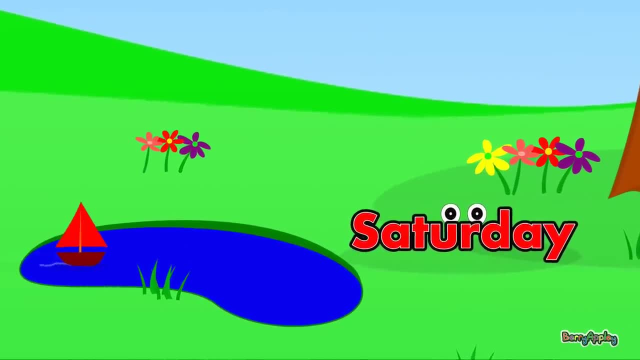 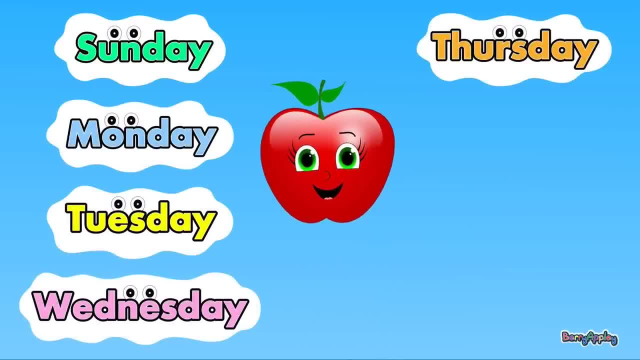 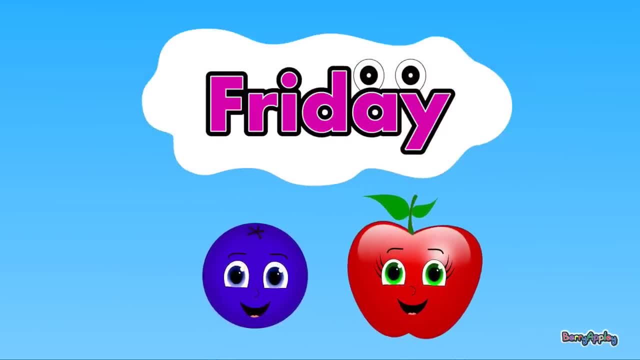 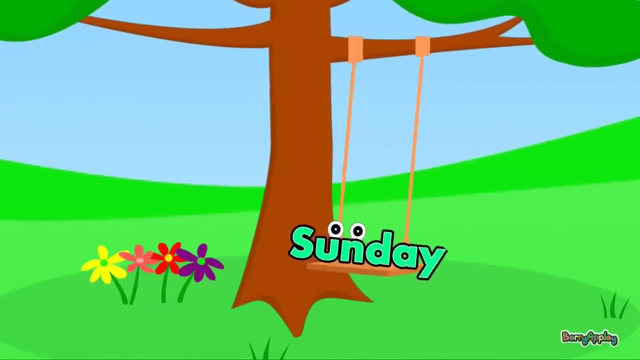 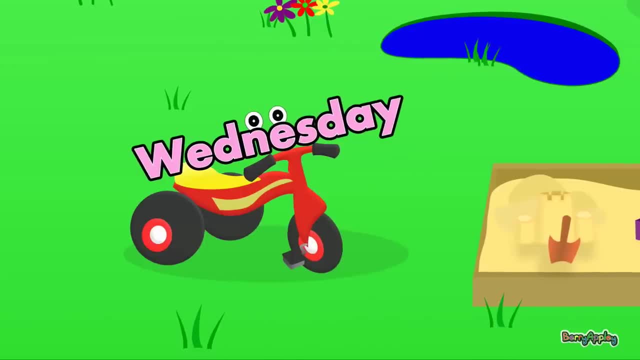 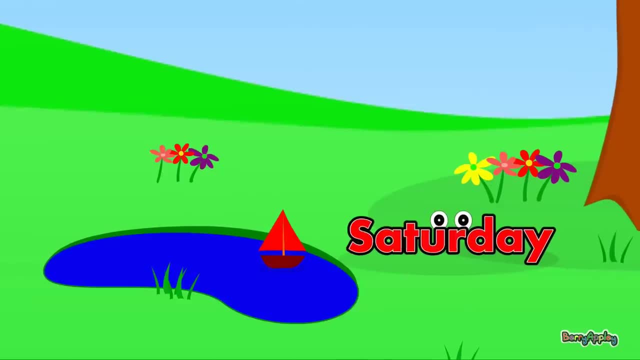 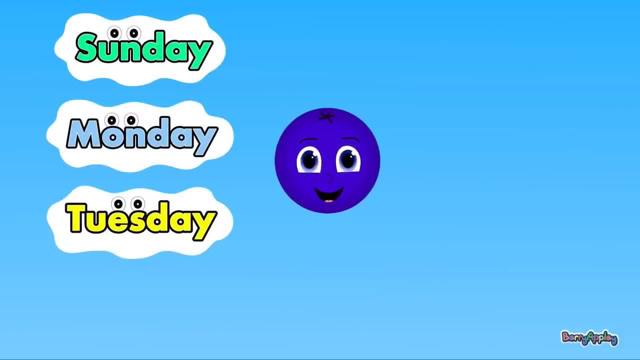 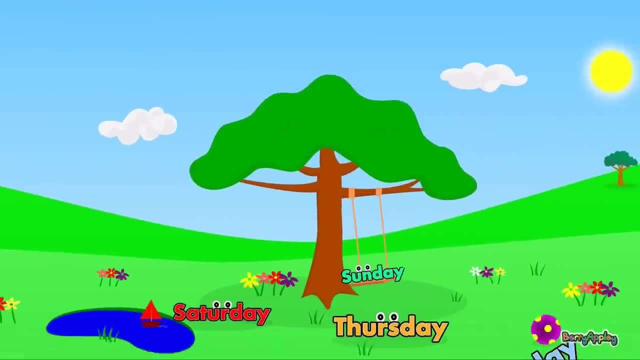 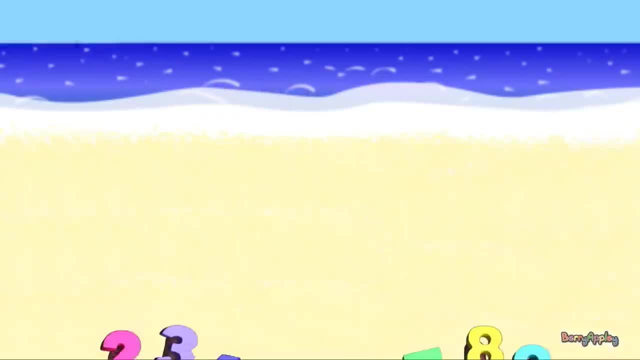 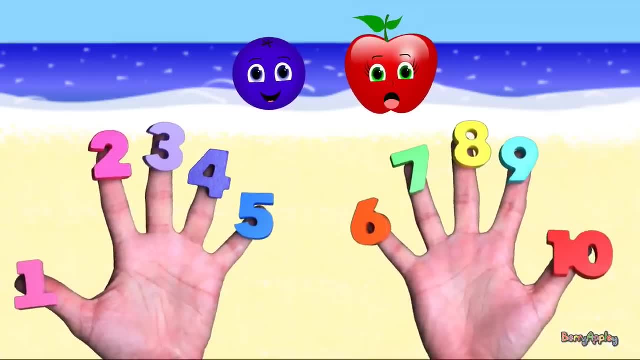 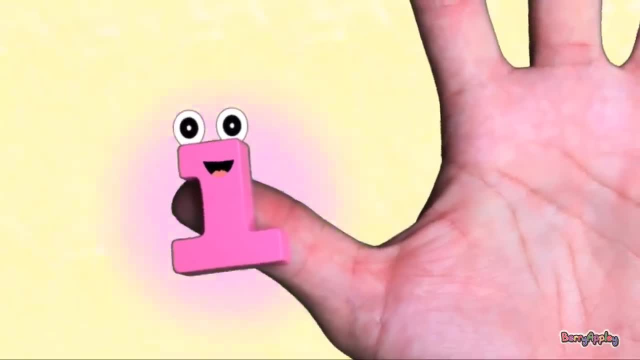 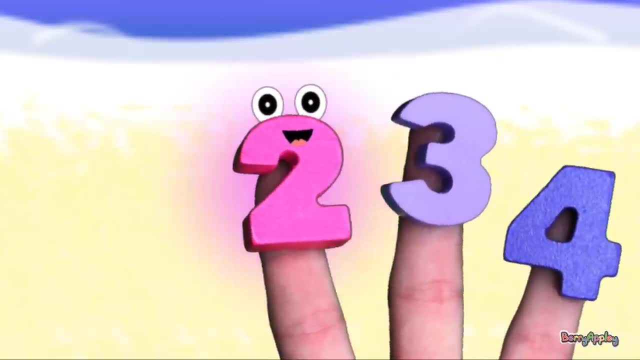 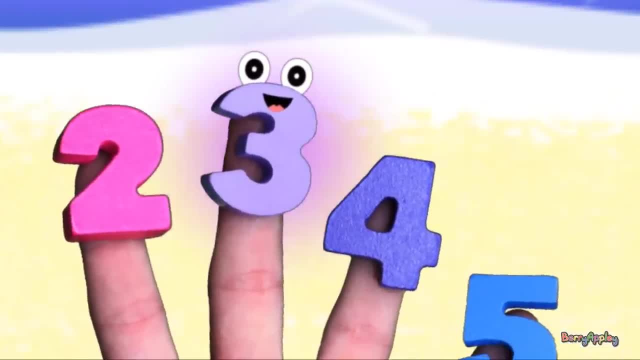 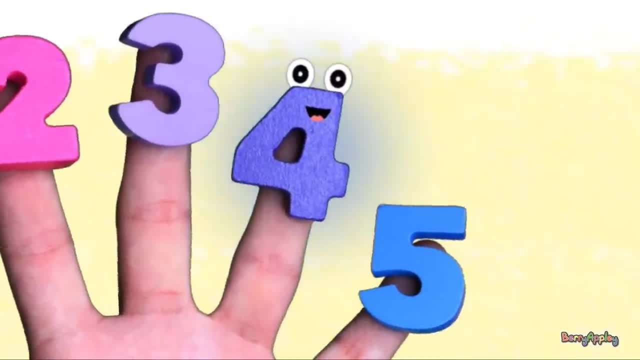 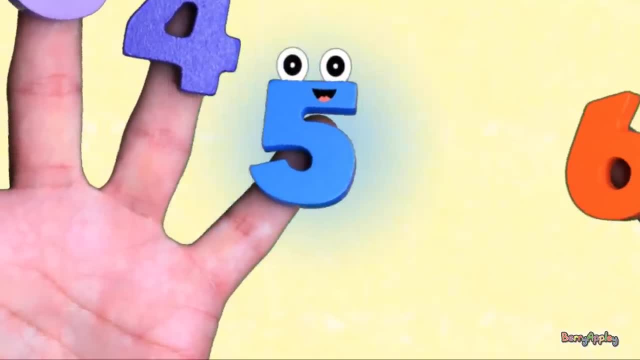 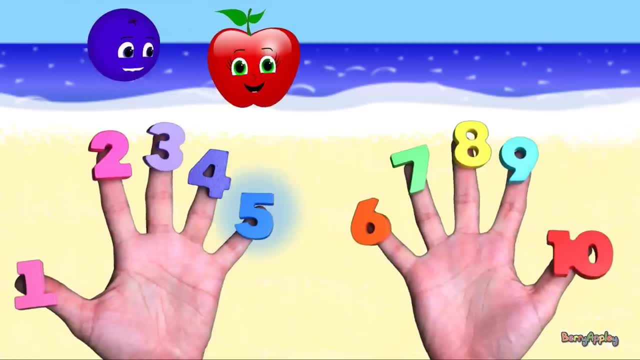 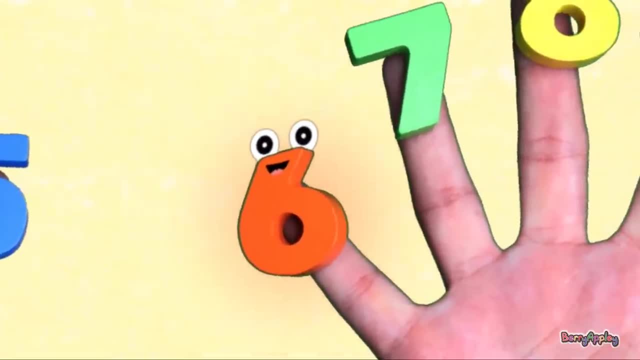 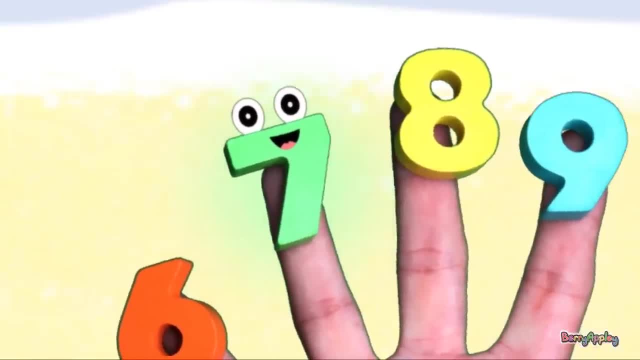 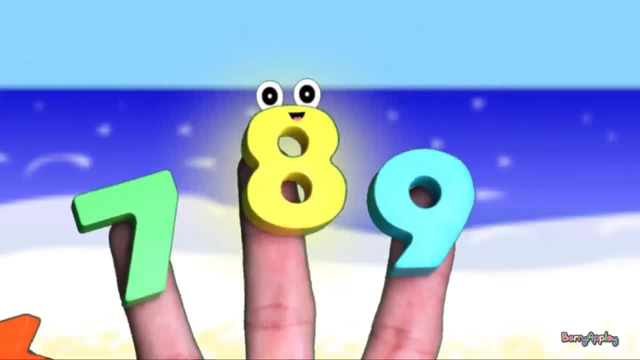 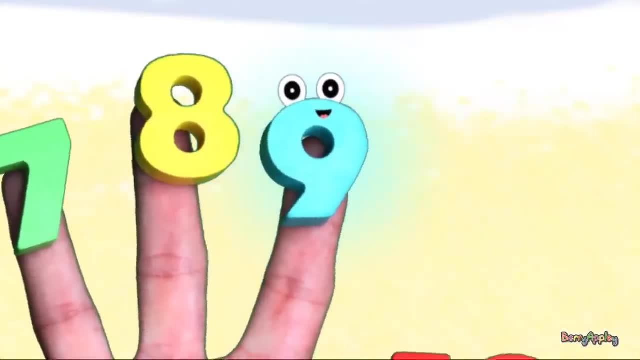 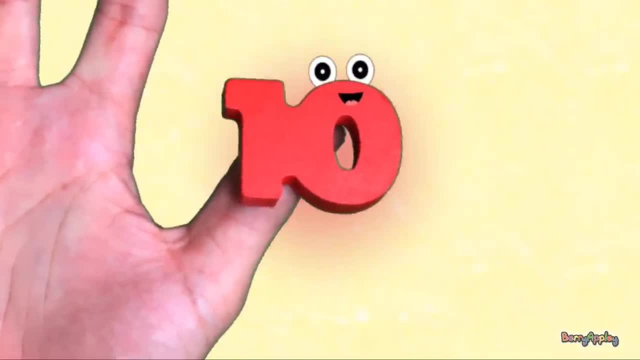 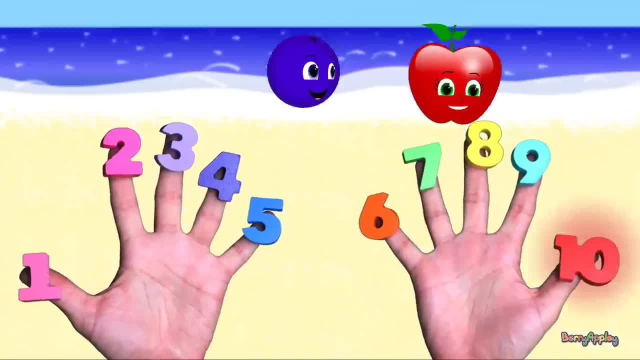 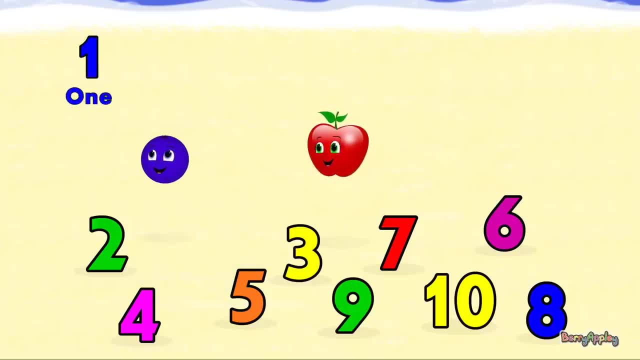 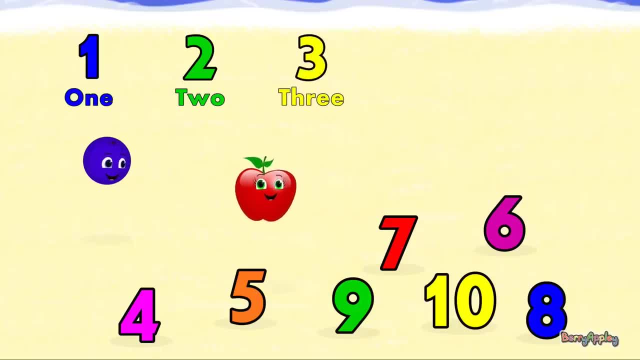 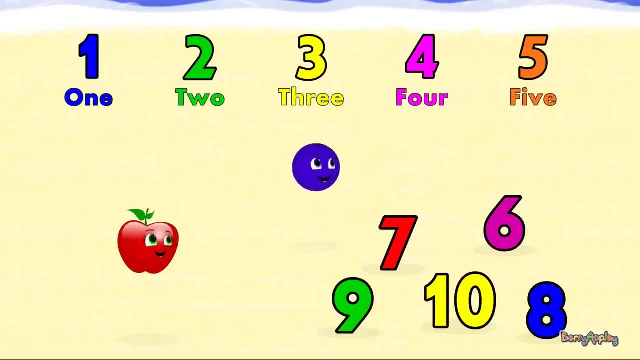 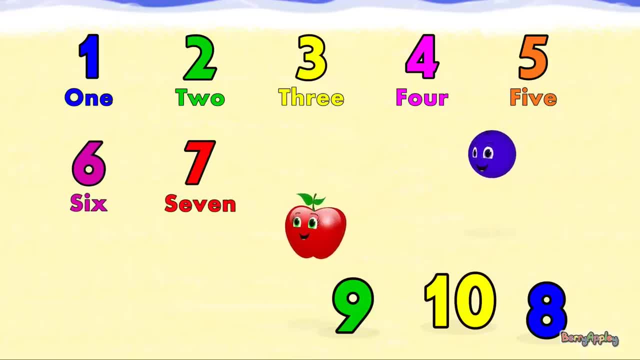 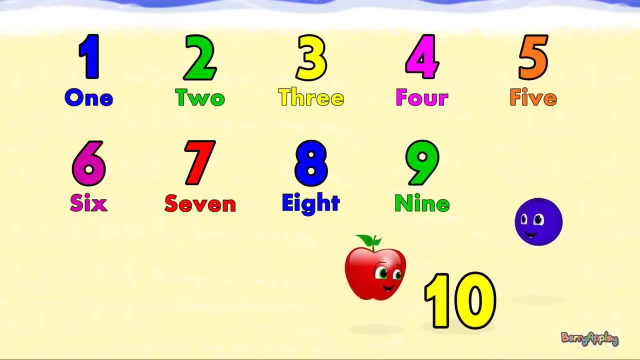 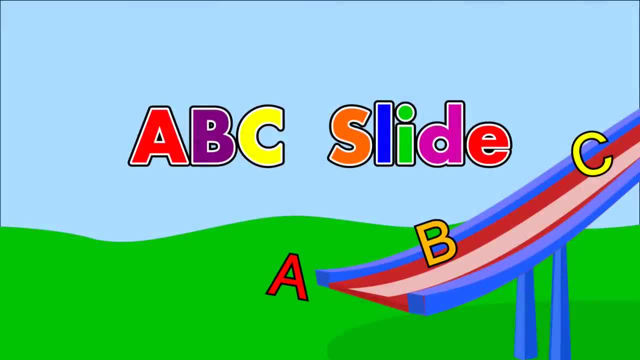 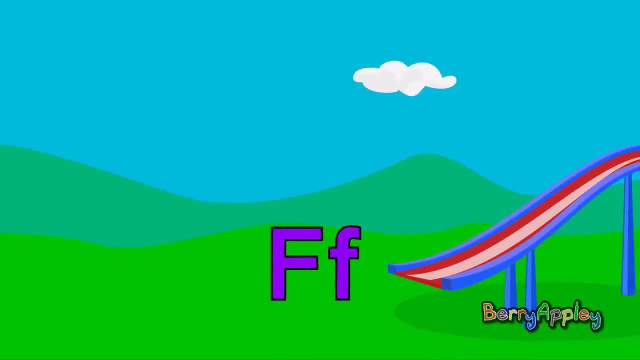 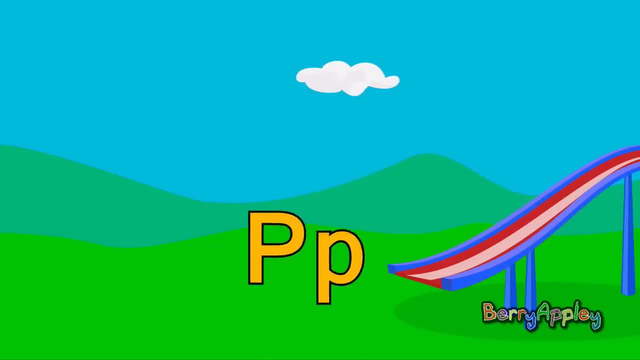 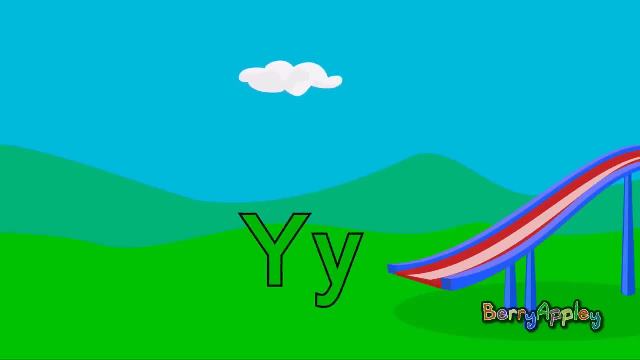 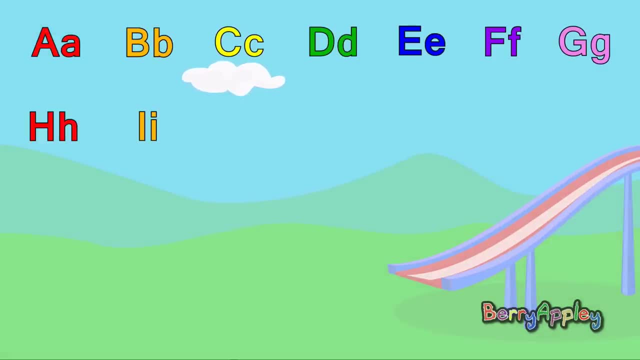 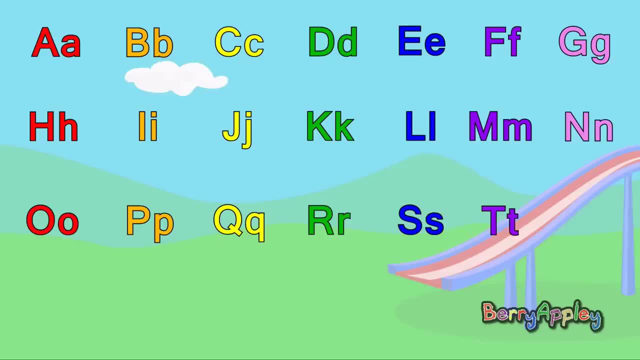 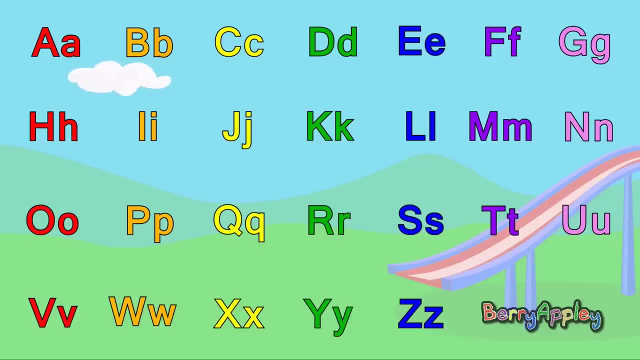 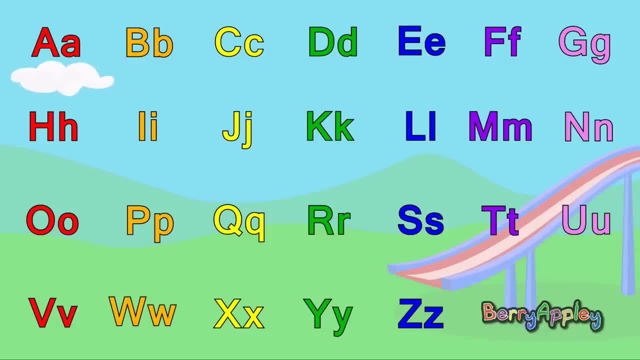 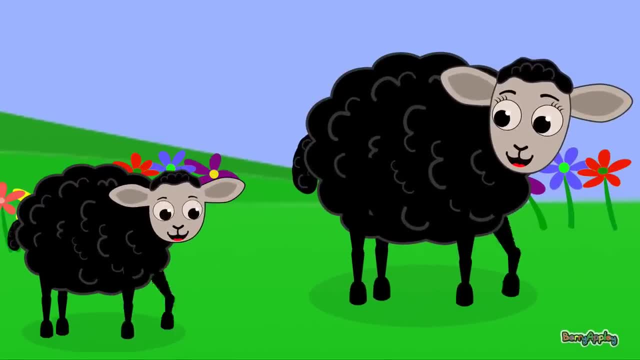 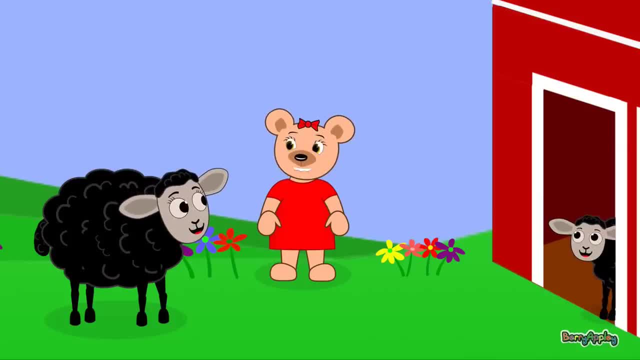 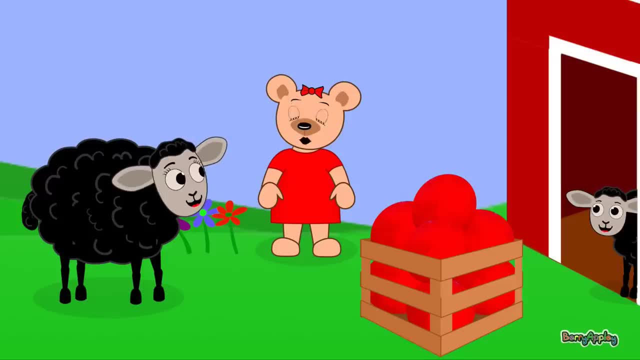 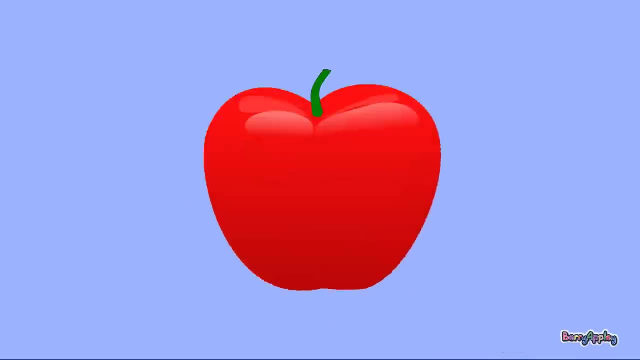 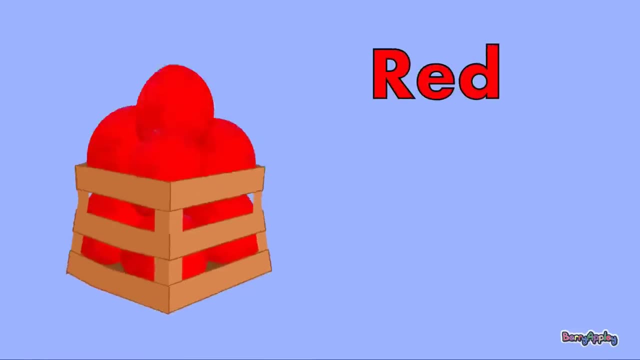 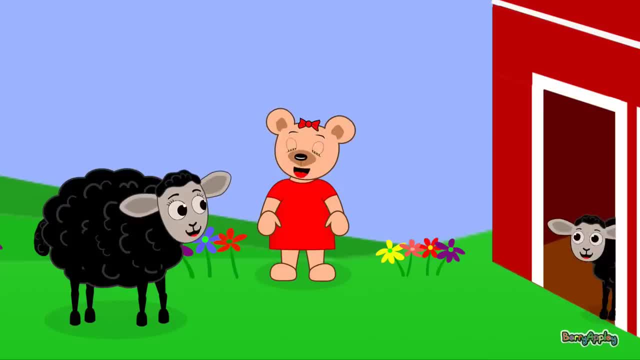 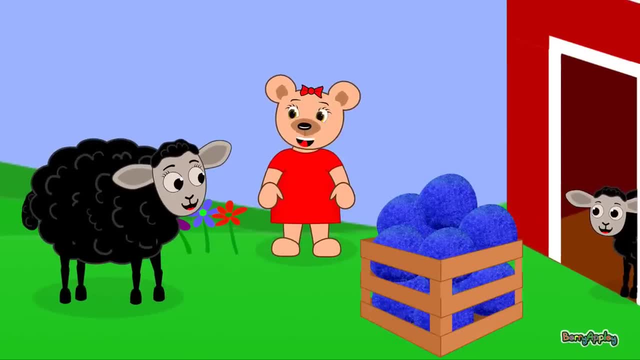 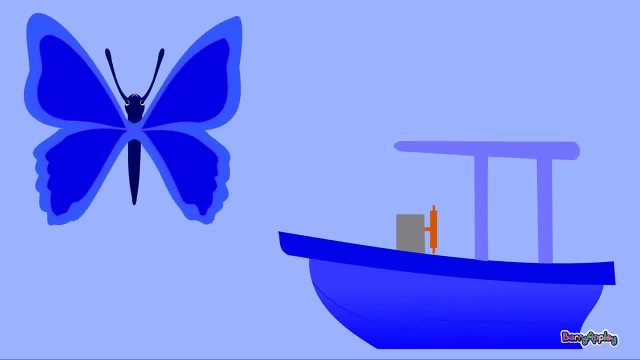 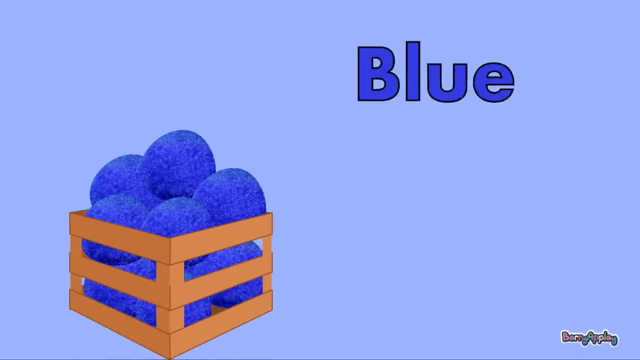 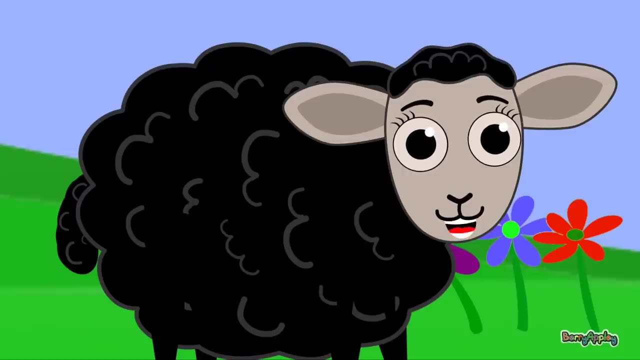 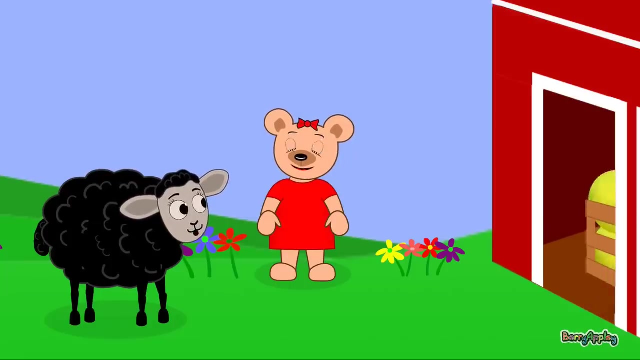 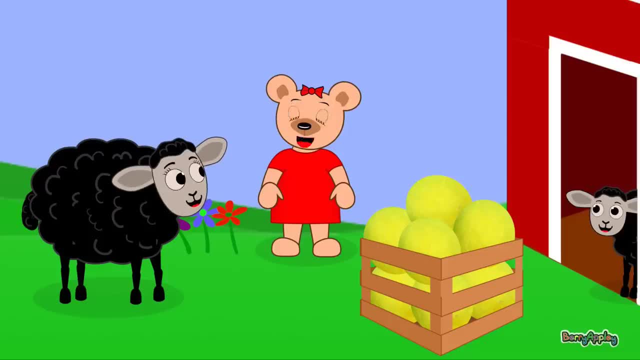 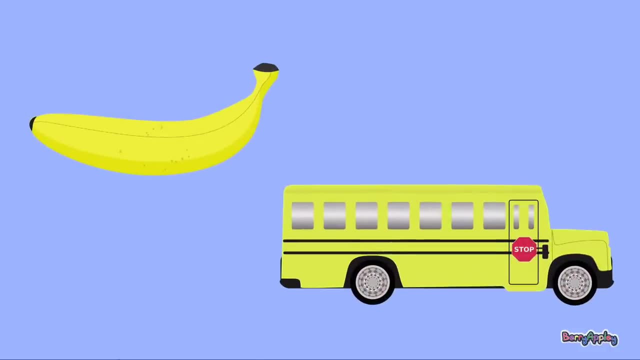 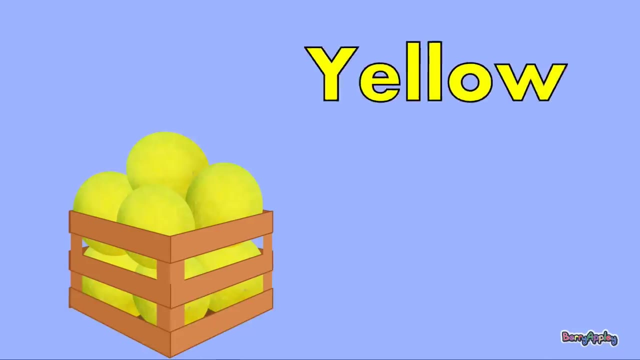 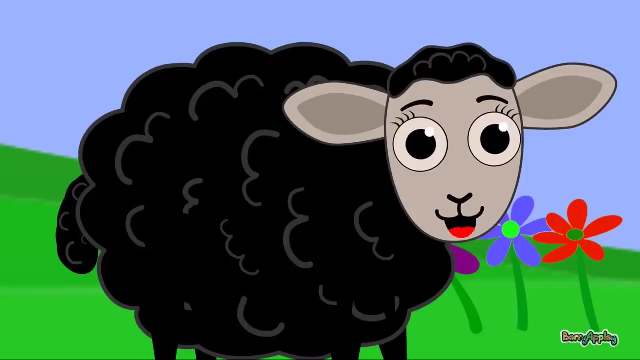 Can you tell me something's not a yellow, Yellow, banana yellow bus. those are yellow, Yellow, banana, Yellow bus. Can you say: yellow, Yellow, yellow. Great job, Baa baa black sheep. do you have green? 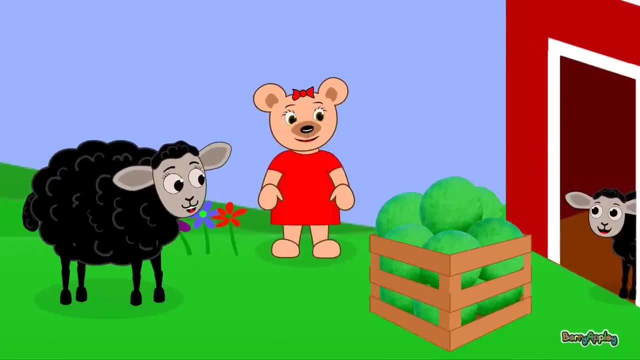 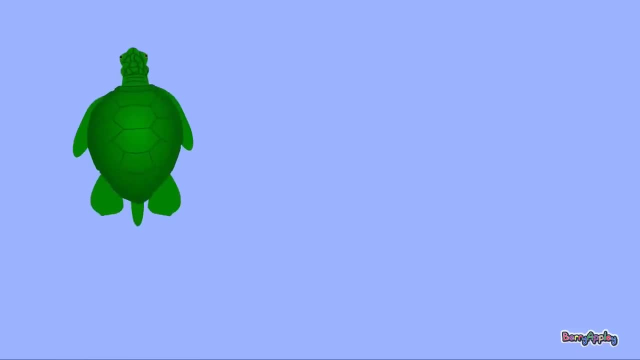 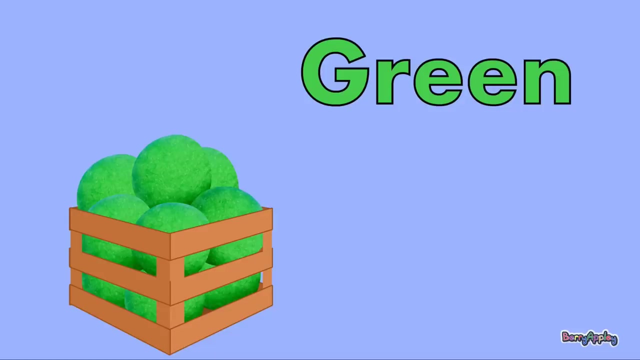 Yes, I do, yes, I do, I have green. Can you tell me something's not a green Green turtle green tree? those are green Green turtle green tree. can you say green, Green, green? great job. 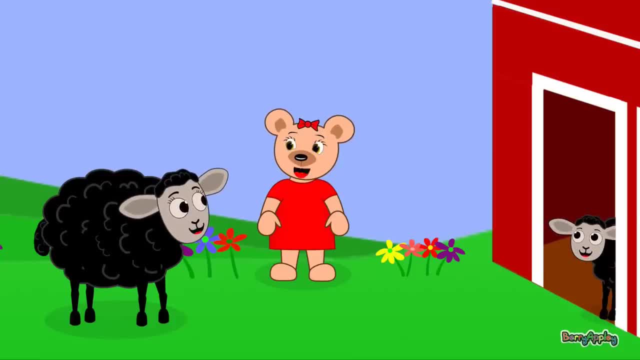 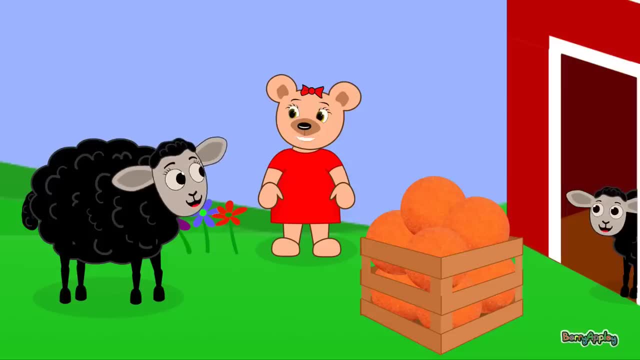 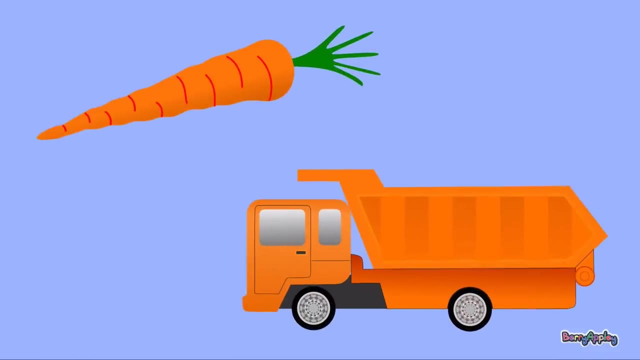 Baa baa black sheep. do you have orange? Yes, I do. yes, I do, I have orange. Can you tell me something's not a orange, Orange, carrot, orange truck. those are orange, Orange, carrot, orange truck. can you say orange? 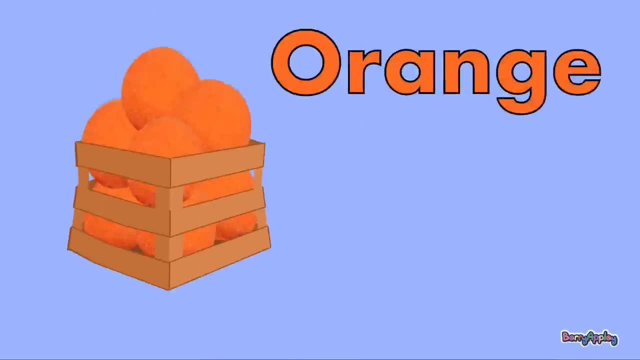 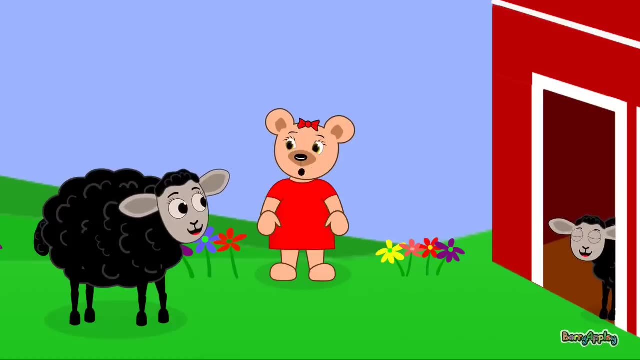 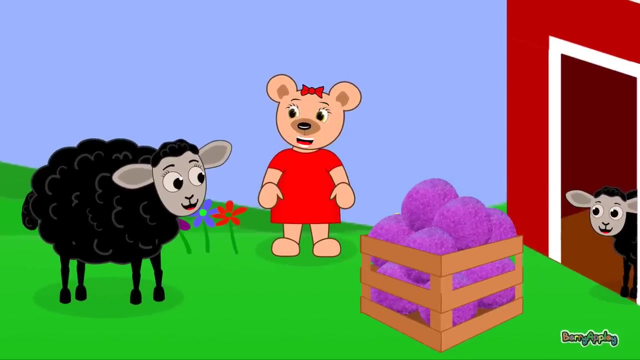 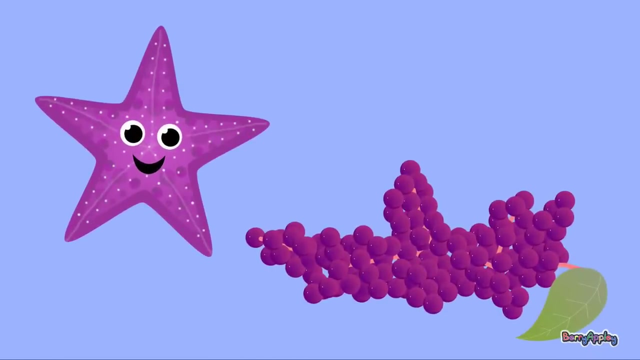 Orange, orange, very good, Baa baa black sheep, do you have purple? Yes, I do. yes, I do, I have purple. Can you tell me something's not a purple, Purple starfish, purple grapes, those are purple. 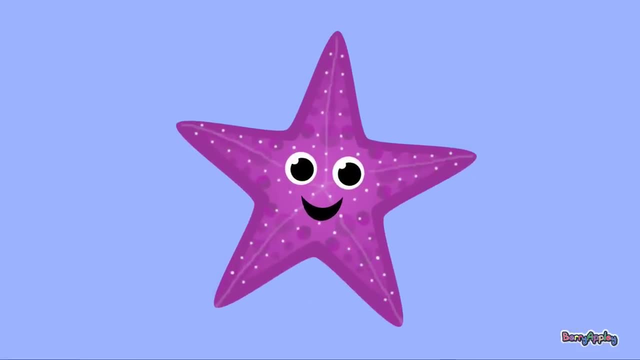 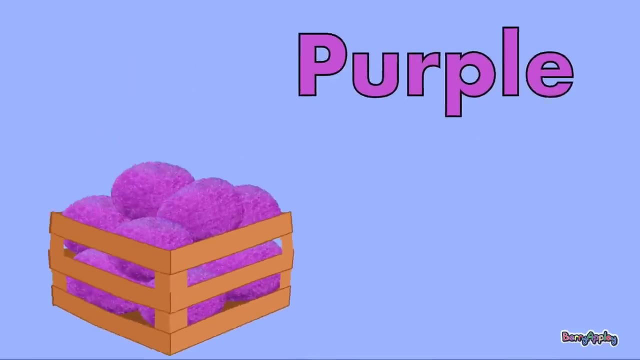 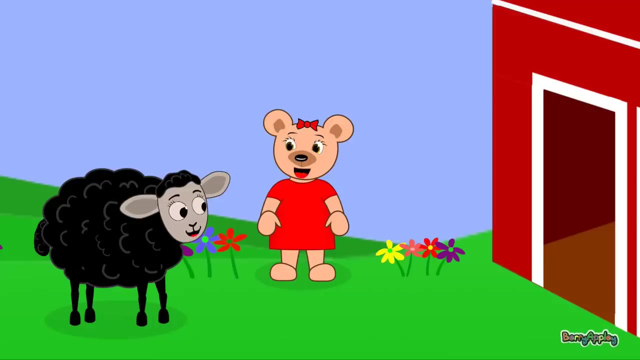 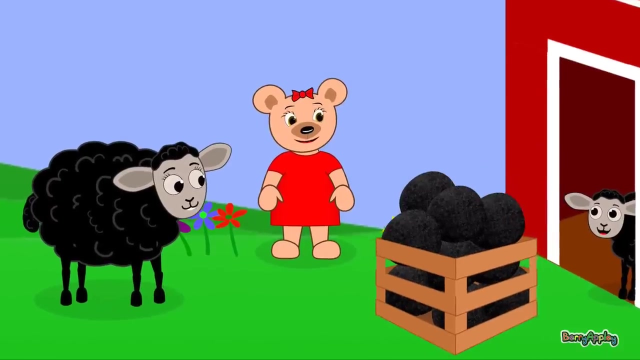 Purple starfish, purple grapes. can you say purple, Purple, purple. good job Baa baa black sheep. do you have green? Do you have black? Yes, I do. yes, I do, I have black. 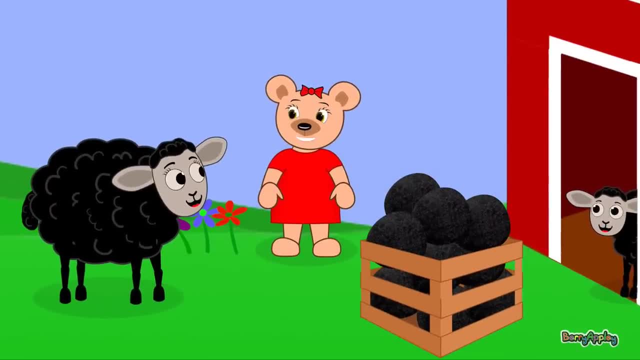 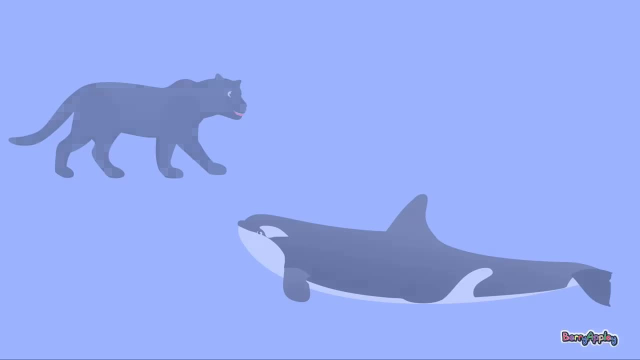 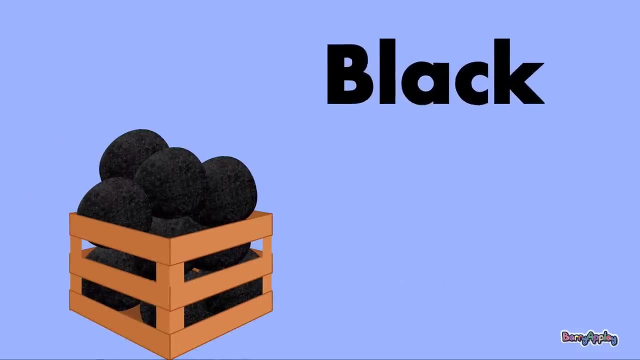 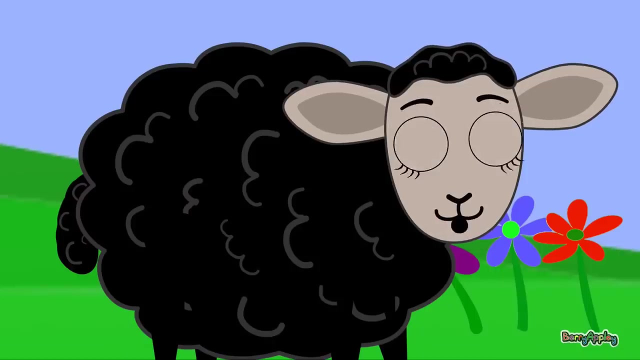 Can you tell me something's not a black Black panther, black orca. those are black Black panther, black orca. can you say black Black, black? Very good, Baa baa black sheep. do you have gray? 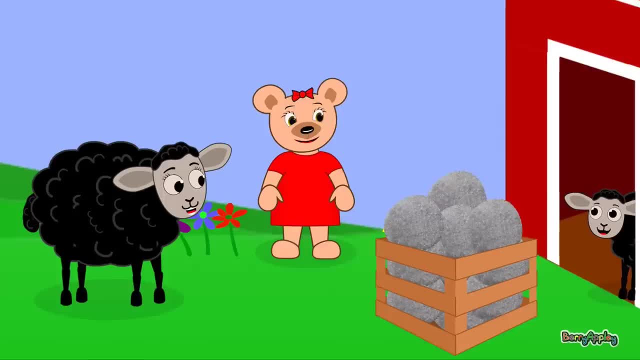 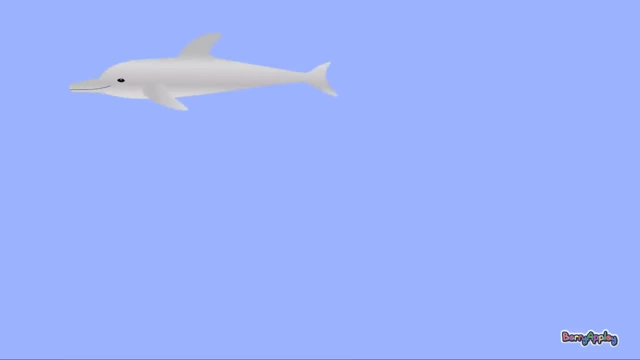 Yes, I do, yes, I do. I have gray. Can you tell me something's? not a gray Gray dolphin, gray donkey? those are gray Gray dolphin gray donkey. can you say gray, Can you say gray? 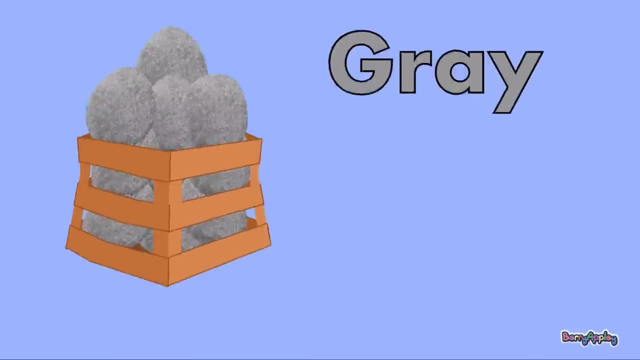 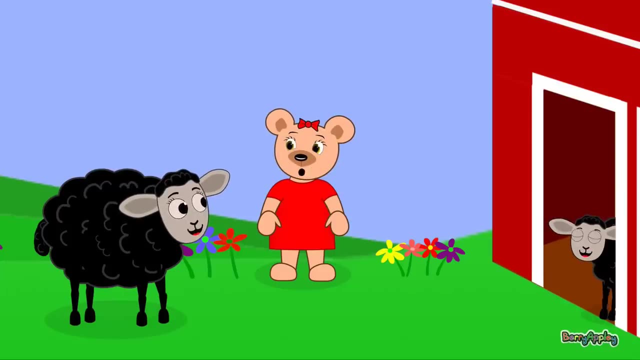 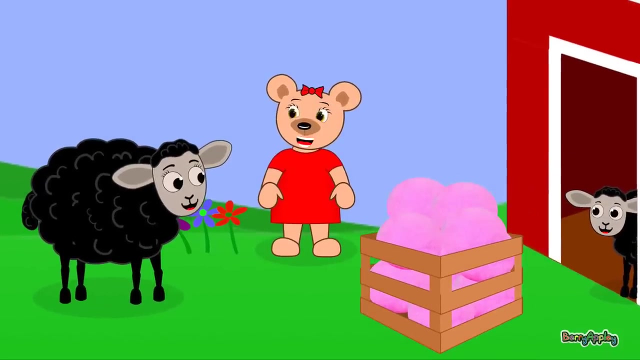 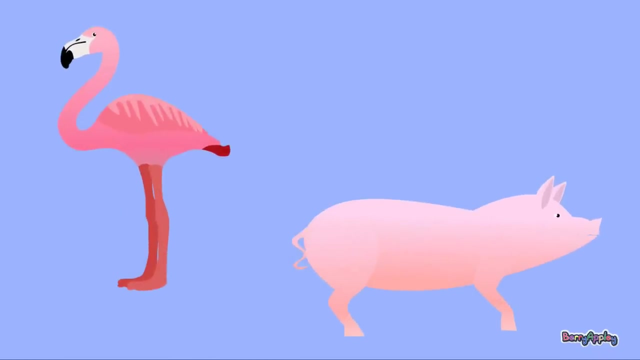 Gray gray. very good Baa baa black sheep, do you have pink? Yes, I do. yes, I do, I have pink. Can you tell me something's not a pink, Pink flamingo, pink pig, those are pink. 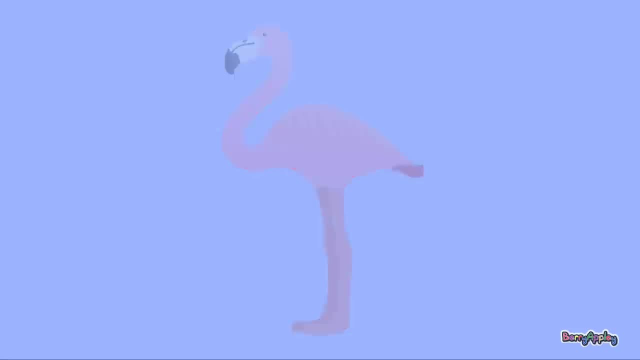 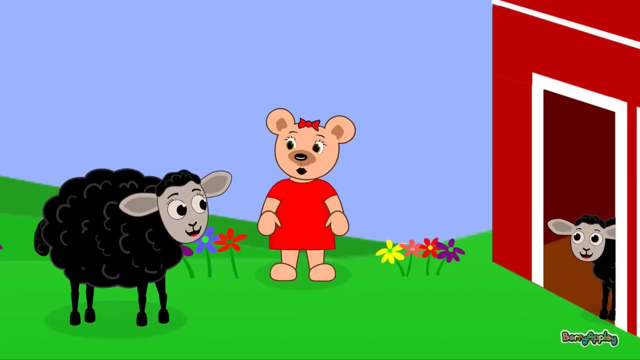 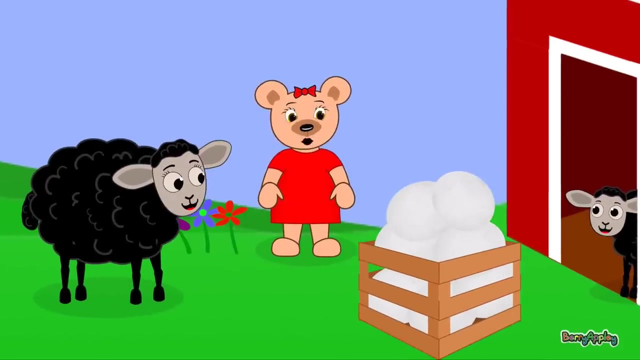 Pink, flamingo, pink pig. can you say pink, Pink, pink. good job Baa baa black sheep. do you have white? Yes, I do. yes, I do, I have white. Can you tell me something's not a white?